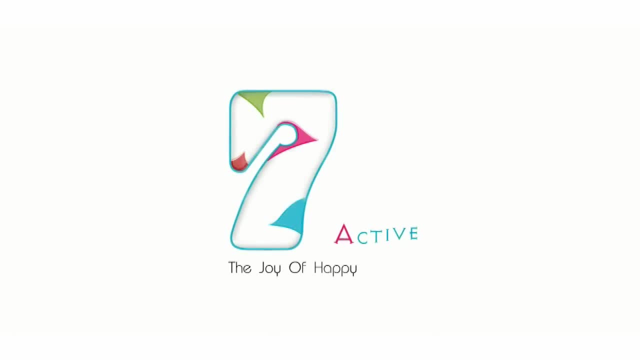 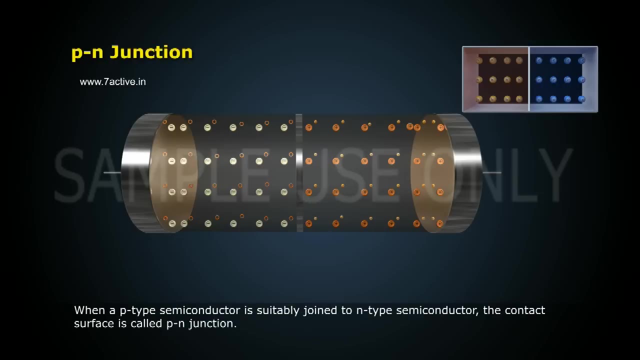 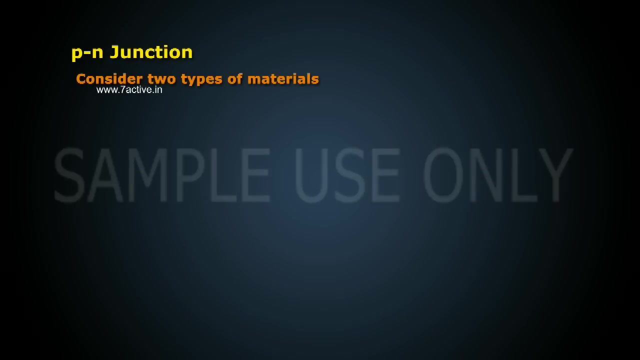 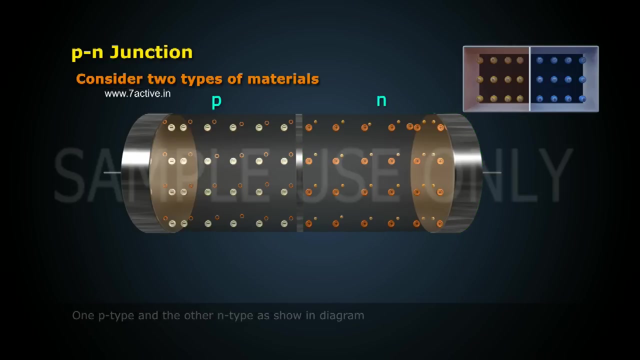 P-N junction. When a P-type semiconductor is suitably joined to N-type semiconductor, the contact surface is called P-N junction. Consider two types of materials: One P-type and the other N-type. as shown in diagram Left side material is a P-type semiconductor. 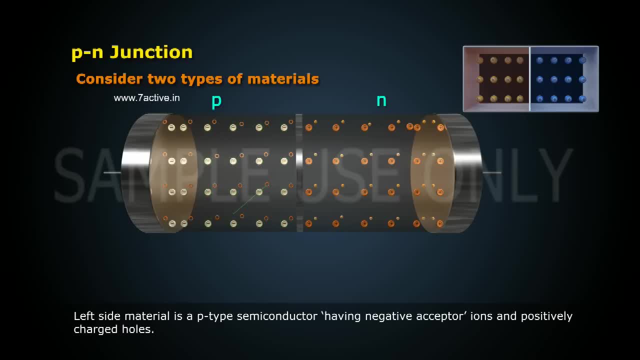 having negative acceptor ions and positively charged holes. The right side material is N-type semiconductor having positive donor ions and free electrons, Suppose the two pieces are suitably treated to form P-N junction. Keep in mind that N-type material has a high concentration. 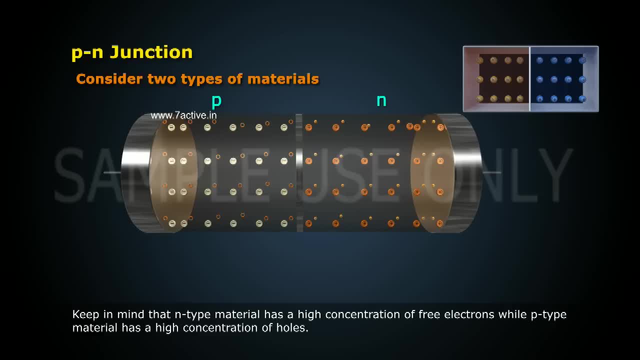 of free electrons, while P-type material has a high concentration of holes. Therefore, at the junction there is a tendency for the free electrons to diffuse over to the P-side and holes to the N-side As the free electrons move across the junction from N-type to P-type. 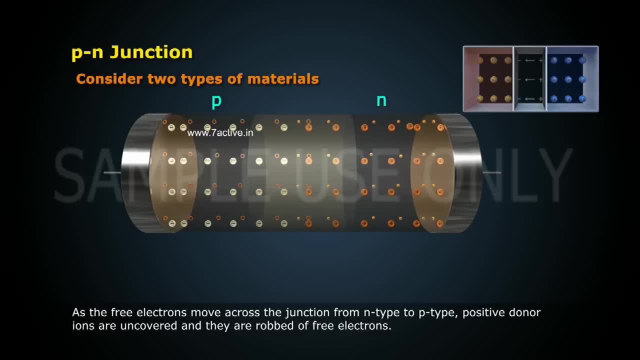 positive donor ions are uncovered and they are robbed of free electrons. Hence a positive charge is built on N-side of the junction. At the same time, the free electrons cross the junction. Therefore an N-type metal in the N-type Parlament about the negative acceptor ion is discovered and the holes are. 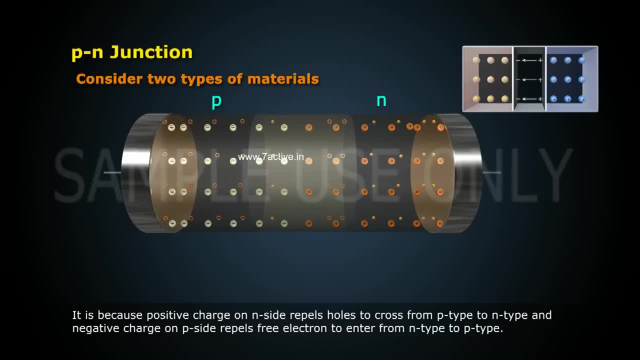 filled in the negative acceptor ions separately. The negativehueltude of the unpaired receptor through the P-typeional is called the NAU and is normally separated by negativeurons due to three Carterl terms: A negative charge through this foreign microstructure tube which is called the crucian. The negative charge on the N-type nectarine. George Byron' conditions are not 동 tactileㅎ.